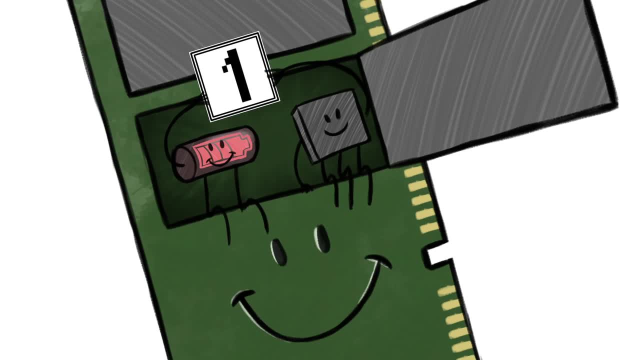 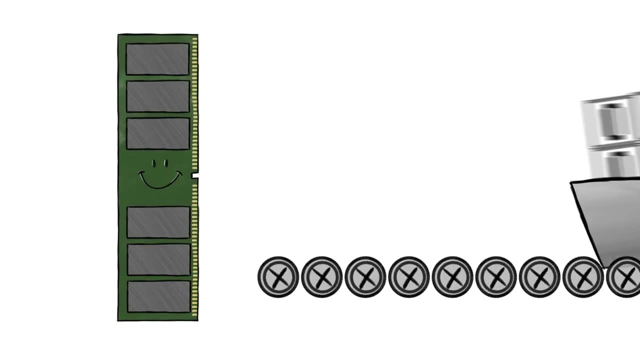 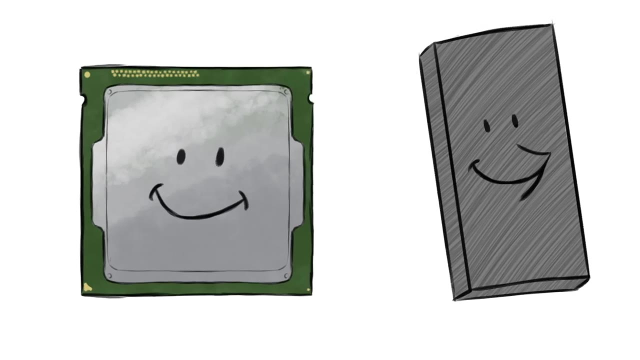 Such memory is called dynamic because it only holds charges briefly before they leak away, requiring periodic recharging to retain data. But even its low latency of 100 nanoseconds is too long for modern CPUs, So there's also a small high-speed internal memory cache. 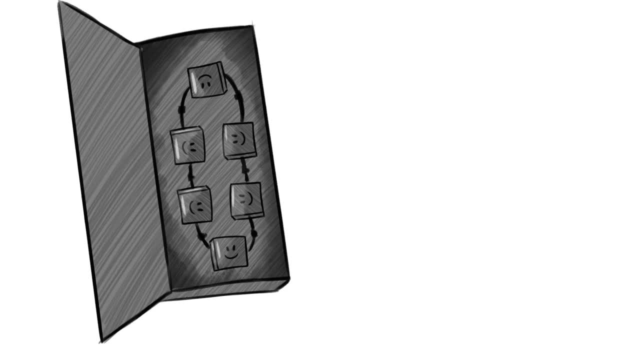 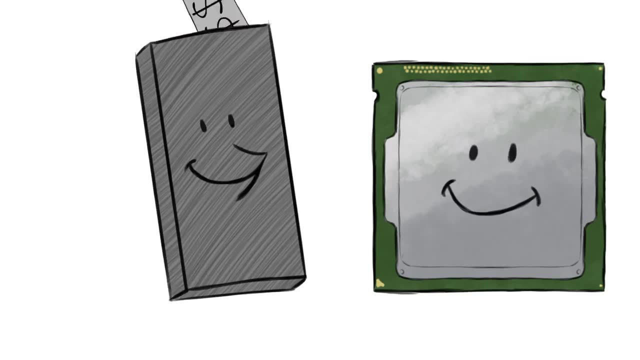 made from static RAM. It's usually made up of six interlocked transistors which don't need refreshing. SRAM is the fastest memory in a computer system but also the most expensive and takes up three times more space than DRAM. But RAM and cache can only hold data as long as they're powered. For data to remain once the device is turned off, it must be transferred into a long-term storage device, which comes in three major types. In magnetic storage, which is the cheapest? 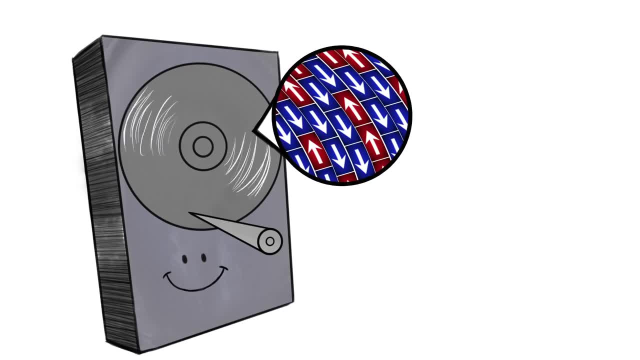 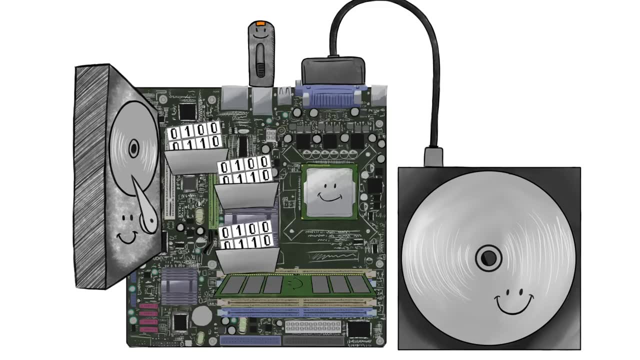 data is stored as a magnetic pattern on a spinning disk coated with magnetic film, But because the disk must rotate to where the data is located in order to be read, the latency for such drives is 100,000 times slower than that of DRAM. 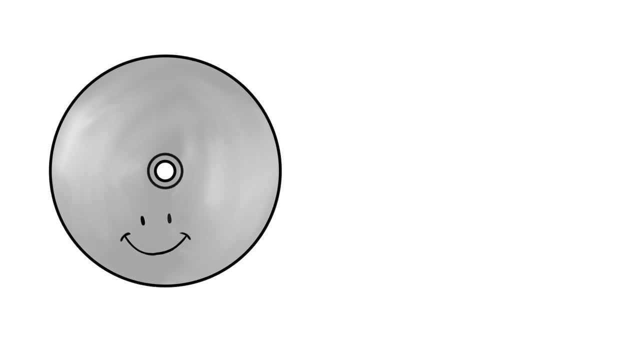 On the other hand, optical-based storage, like DVD and Blu-ray, also uses spinning disks, but with a reflective. coating. Bits are encoded as light and dark spots using a dye that can be read by a laser. While optical storage media are cheap and removable, 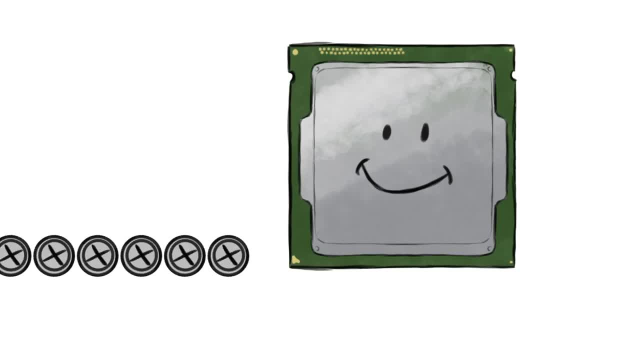 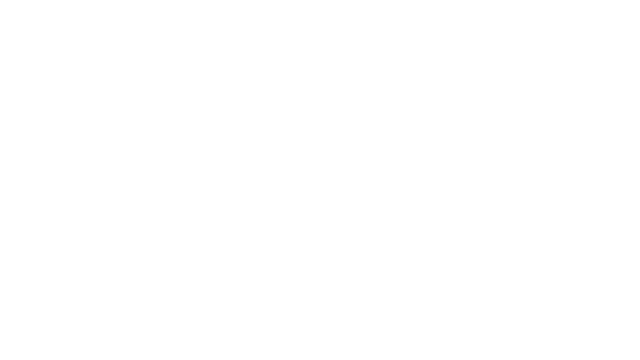 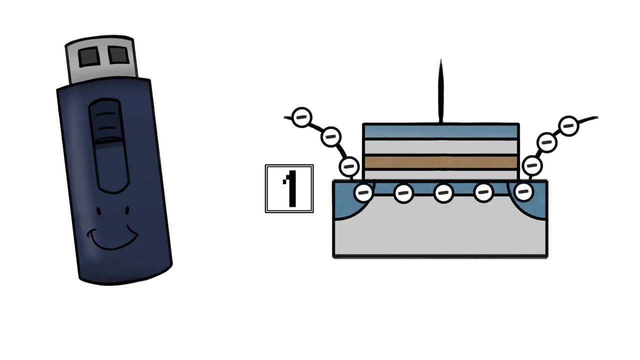 they have even slower latencies than magnetic storage and lower capacity as well. Finally, the newest and fastest types of long-term storage are solid-state drives like flash sticks. These have no moving parts. instead, using floating-gate transistors that store bits by trapping or removing electrical charges, 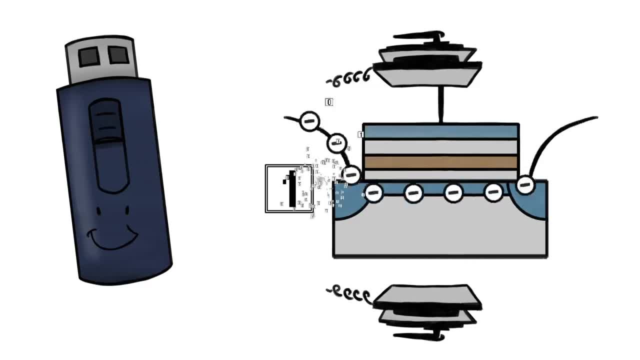 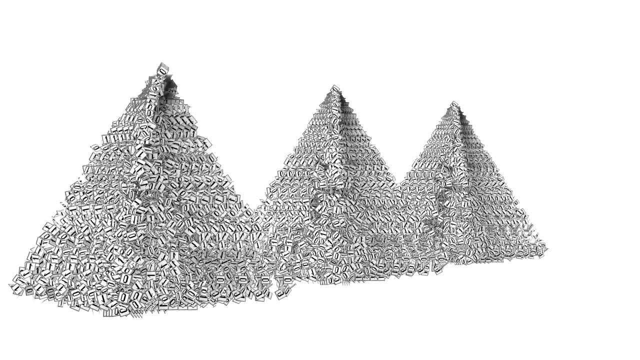 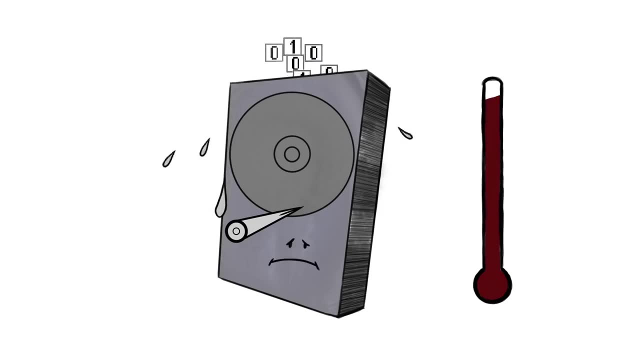 within their specially designed internal structures. So how reliable are these billions of bits? We tend to think of computer memory as stable and permanent, but it actually degrades fairly quickly. The heat generated from a device and its environment will eventually demagnetize hard drives. 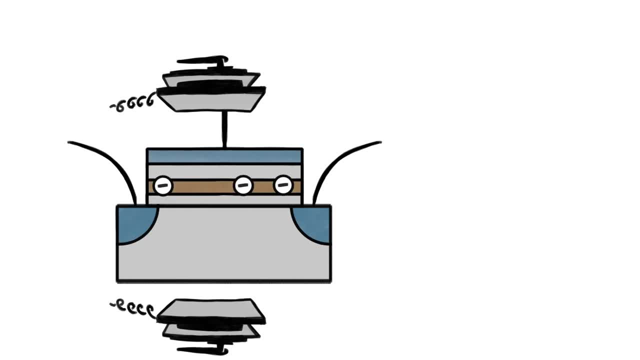 degrade the dye in optical media and cause charge leakage in floating gates. Solid-state drives also have an additional weakness. Repeatedly writing to floating-gate transistors corrodes them, eventually rendering them useless. With data on most current storage media,